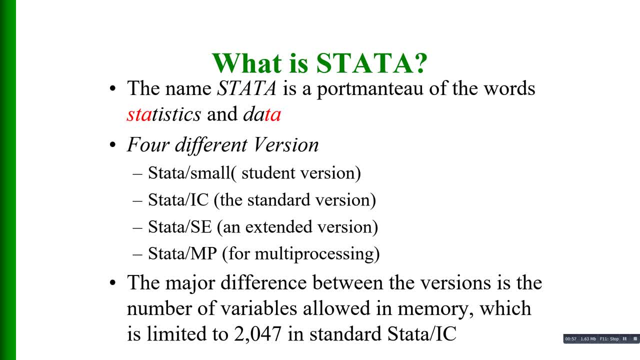 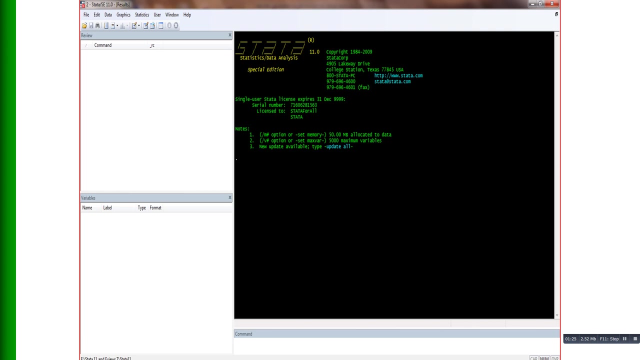 There are four different versions of Stata. One is small, that is called Stata Student version. Then there is Stata IC, that is the standard version, And then there is Stata extended version And, lastly, there is Stata MP for multiprocessing. The major difference between the versions is that the number of variables allowed in memory, which is limited to 2004, to 7. and standard Stata IC. This is how Stata looks like when you initially 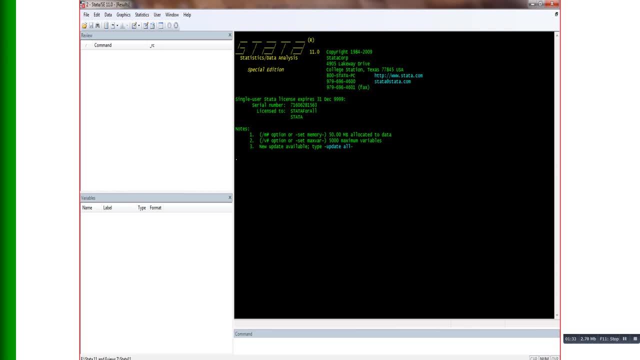 open it. So there are four windows here. Here is the command window. Here is the variable window. Sorry, this is the review window And here will be the list of variables And there will be. this is the command area And here you will see your output. 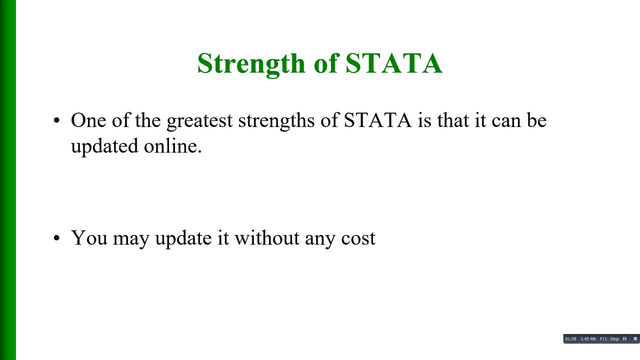 What are the strengths of Stata? One of the greatest. The one of the greatest strengths of Stata is that it can be updated online free of cost. You don't need to pay for it And you may update it without any additional costs. 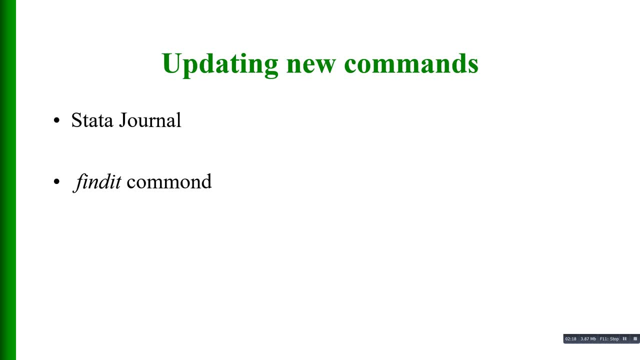 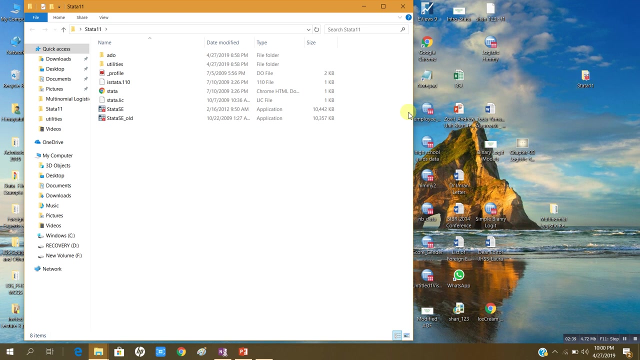 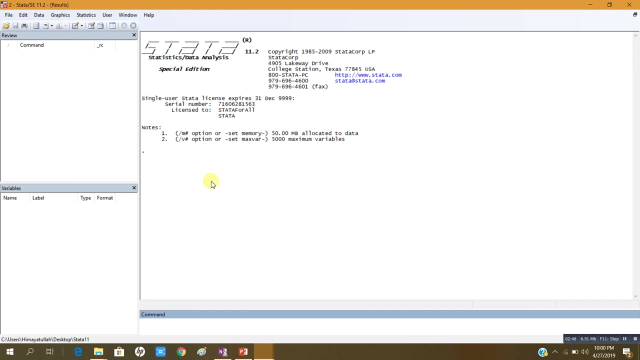 Regarding updating new commands, there is a Stata journal And there is also find it command and you can learn many new commands or you can see updated commands in Stata. Let me just click on state icon in my laptop and you see, here are the four windows. that is the review. 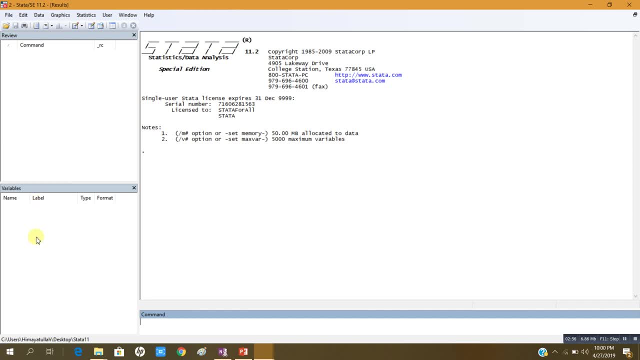 the review window. here will be list of variables and this is the command window where we execute commands, and this is the output area. ladies and gentlemen, you see there is no file in memory right here in the screen. let me tell you. if you press on file and go to example data sets. 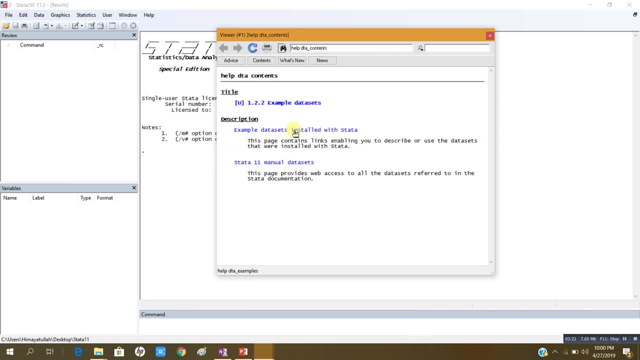 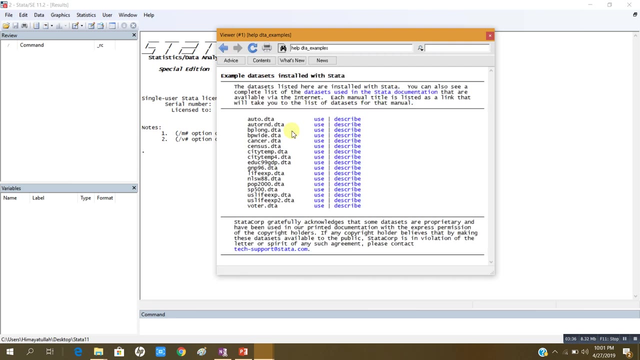 so you can see, there are some data sets which are installed with stata and there are some other manual data sets. so, just for the sake of convenience, let me click on example data sets installed with stata and these are the various types of files which are installed with the stata. dta is the extension for 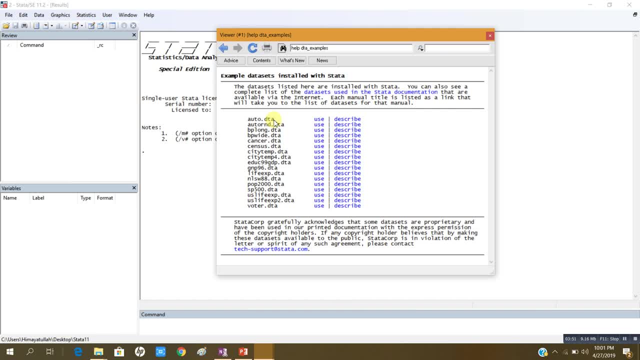 stata file. so these, these are various files which are available online for examples, and we can analyze data from this file. let us suppose i want to open this nlsw8.dta, so i will click on use. so when i click on use, all the variables in this file are listed here, right? so let me check. 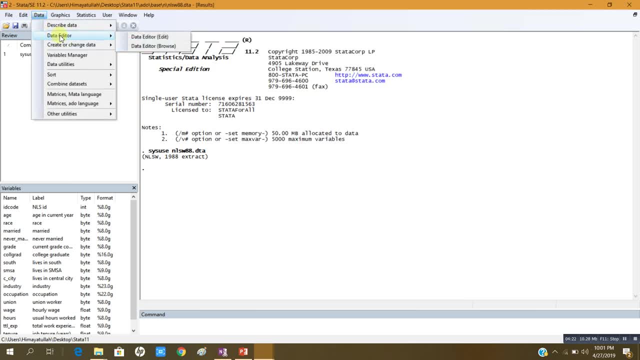 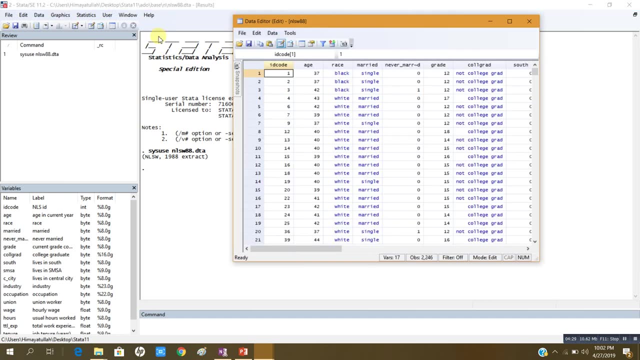 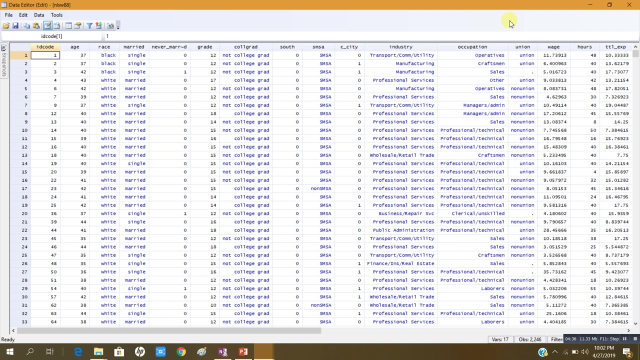 what kind of variables do we have here? so here under data editor, i will go to data editor, edit and if i maximize this, this is: these are the various variables here. now, the first variable here is ID code, the second is age, the third is race, that is, black, white and other, and this is 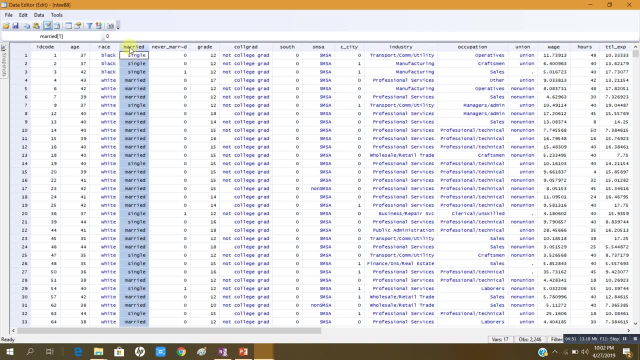 also a categorical variable: married, single. this is never married and this is a great. these are college graduates, college did college graduate and not college graduate and this is dummy for area, South and otherwise. these are some other. these are city and these are the various types of industries. a patient union membership. that is a Union means the subject is a member of the. 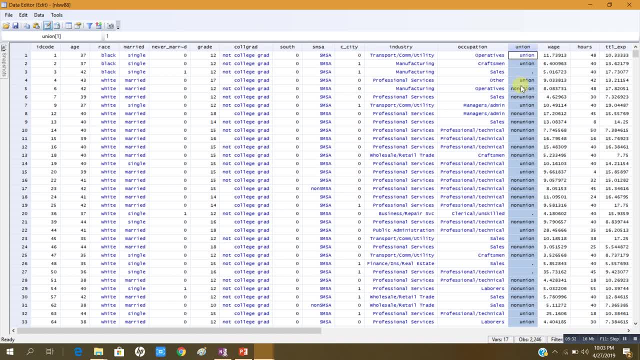 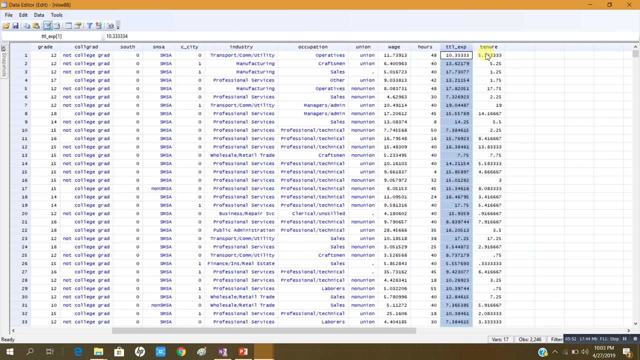 union and the subject is a member of the union. non-union means that the subject is not member of the union and there are some missing cases also in this. this is hourly wage, that is a numeric variable, and this is hours worked and this is total experience in years and this is tenure, job tenure- how many years worked on present job? so 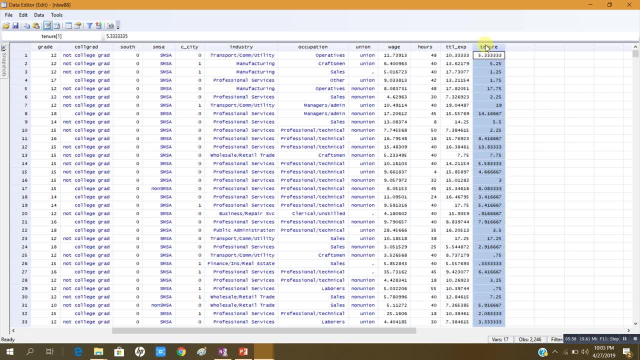 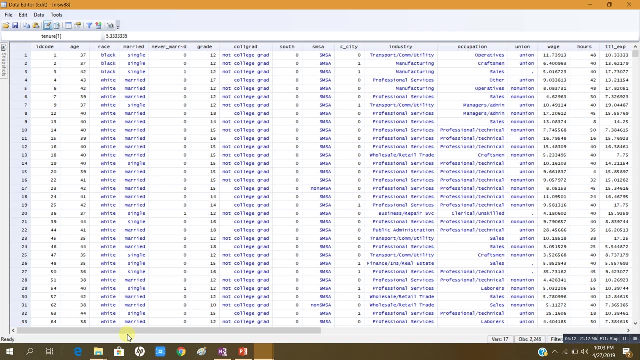 there are a number of variables, some of categorical and some of a numeric, that is, scale variables may be interval or ratio variables. so I start with very basic analysis, since this is my first video in Stata, so let me start with the very basic one and slowly and gradually I'll be. 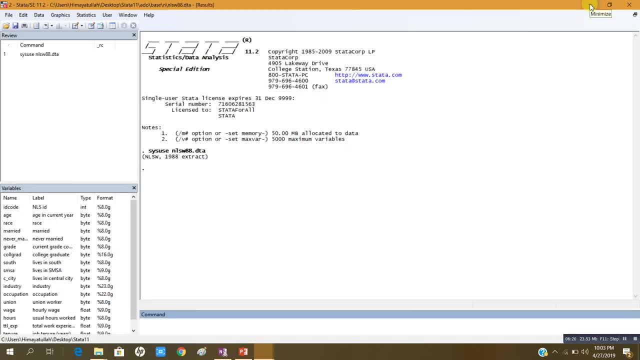 using the advanced analysis. so tonight I am going to start with the very basic frequency distribution, one-way tabulation, a two-way tribulation, that is, cross tapes, multiple cross tapes, coefficient of correlation and simple linear regression. so how can I do that this data is in the memory? 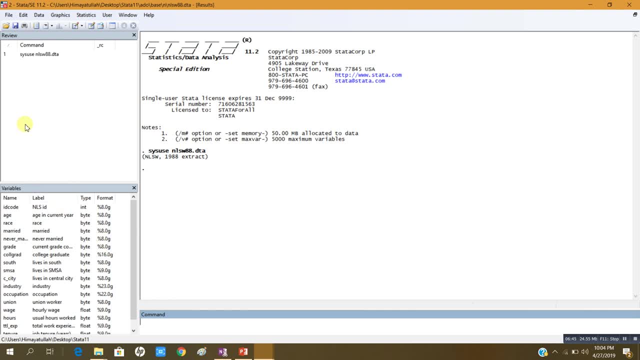 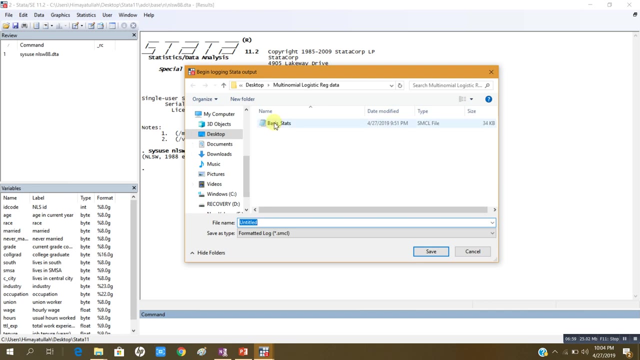 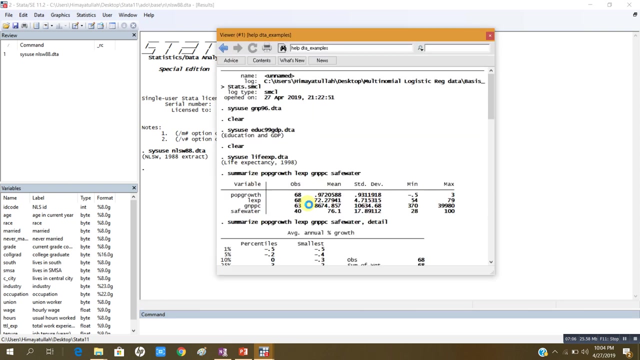 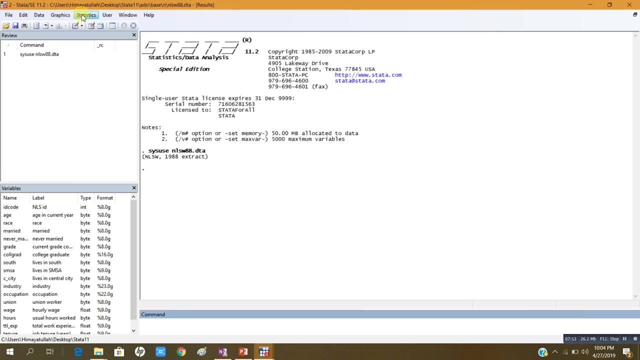 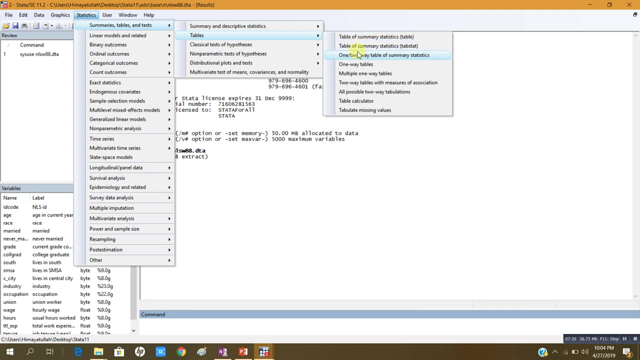 remember. you can always tell the computer to save your work in a log file and let me give it a name: basic state. ok, so it should begin. let me close this now. I want to make some tables, one-way tables. now I start with a very simple one-way table, and one-way table mean: 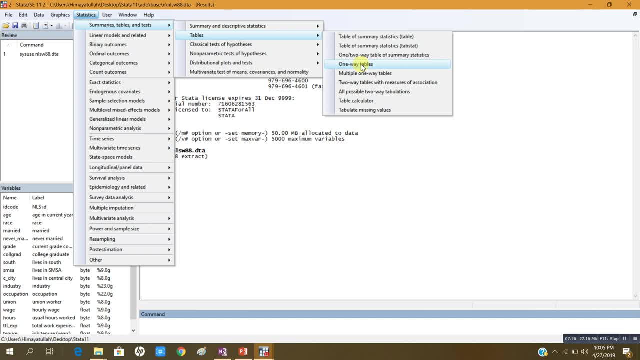 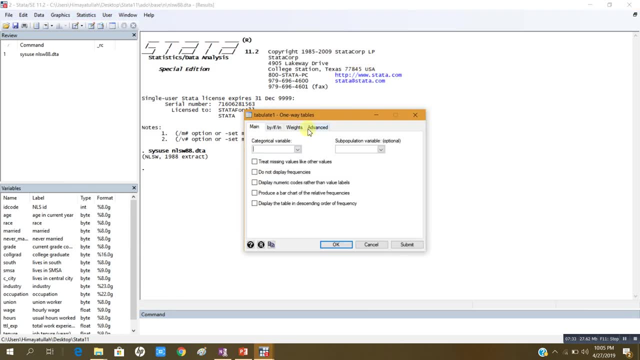 practicing distribution of categorical variables. so if I press that in this dialog box, there are a number of variables now, age is a numeric or scale variable, so I am not going to make frequency distribution of age. but race is a categorical variable and there are two or three categories: black, white and others. let me click on this and let me press ok. if I press ok, 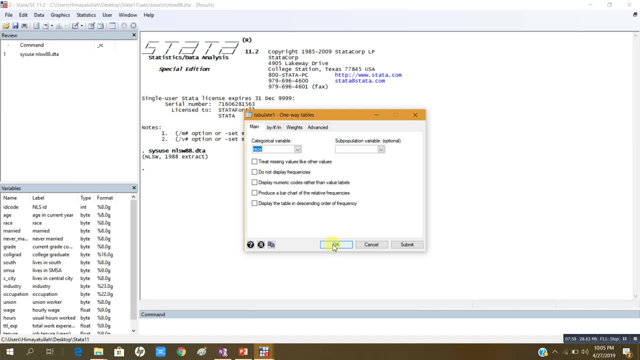 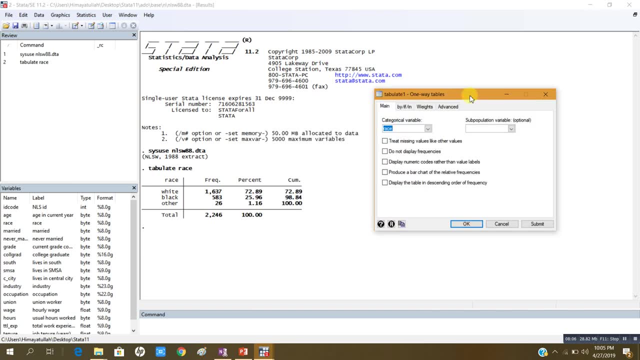 ok, let me submit it so that the command remains here. so here is, I submitted. so here is the frequency distribution of race. you see, there are three categories: white, and the number of white in this category are 1630. 7, which constitutes 72.89% of the total, and the total number of individuals are 2246. 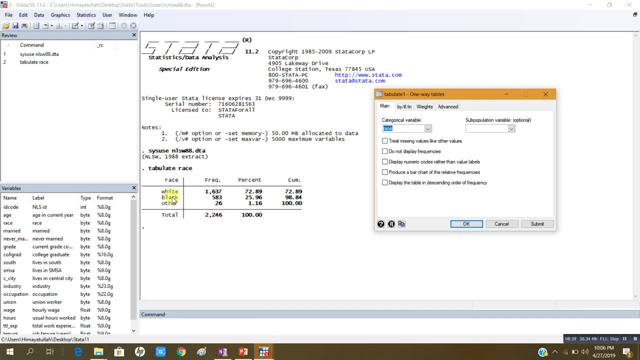 the number of blacks is 483 and it's a percent, is a twenty five point nine. six other are only 26 and it constitutes 1.16 percent of the total. the last column shows the cumulative percentage of the three categories, that is a 72.89, and then if you add 25.98 to 72.89, then it becomes: 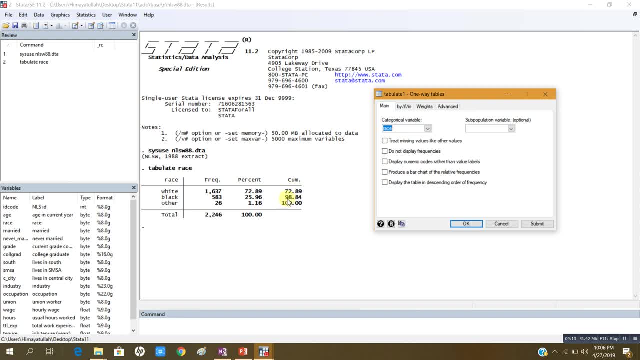 98.84, and if you add at 1.16, then it becomes 100 percent. so that is cumulative percentage. now let me let me, instead of race, let me put merit here, and this time, instead of submit, i press ok. so if i press ok, then this dialog box: 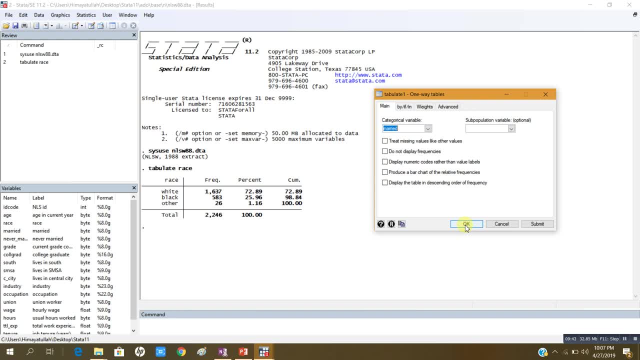 will vanish, but the table will be here. so this is the frequency table of merit, that is the classification of respondents or individuals by marital status. so out of the total 2246, 804 are single and 1442 are married. these are the percentages and these are the cumulative percentages. so let me again repeat this process for another variable. 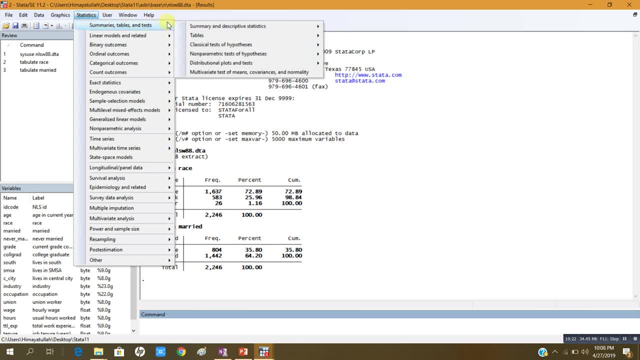 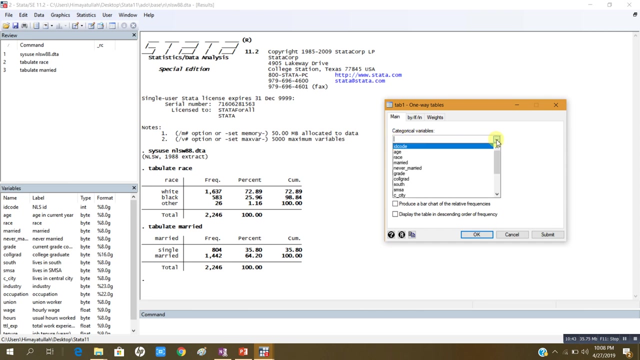 and this time i i want multiple one-way tables instead of making one table. i can make multiple one-way tables at a time, so press this and now i will list the variables. categorical variables, that is race, merit and, say, college graduate. so there are three categorical variables and this time i want to submit. if i press submit, then this dialog box will stay here, but if 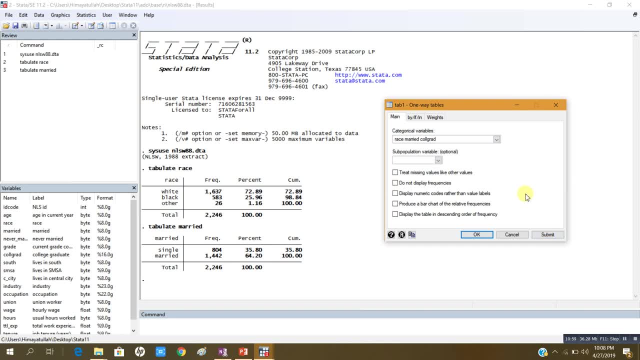 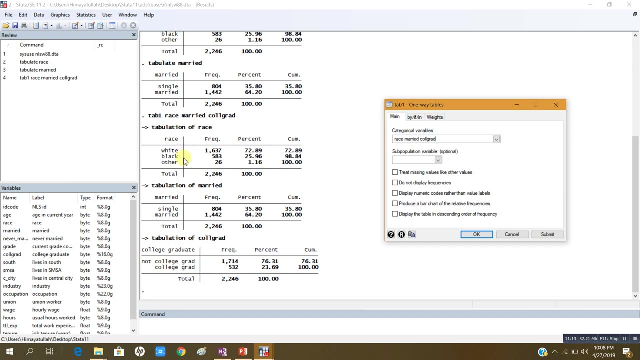 i press ok, then it will disappear and the tables will be here. so i just want to submit, and here are the three one-way tables. since my command was multiple one-way tables, so i listed three variables: one race, married and college graduates. now this table shows that 100, 1637 are white, 583 are black. 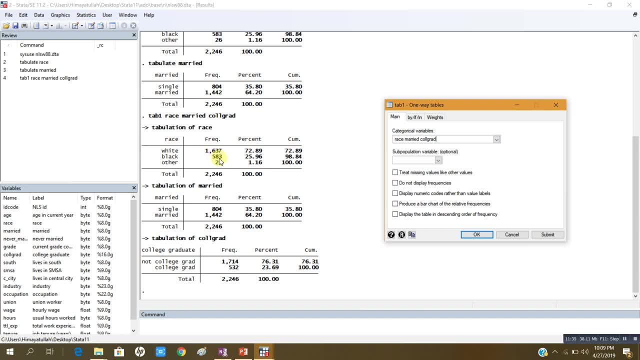 and others constitute 26. the total number of individuals are 2246. these are percentages and these are cumulative percentages. similarly, in this table, this is classification of total individuals by marital status: 804 are single, 1442 are married. it means 64 percent are married and 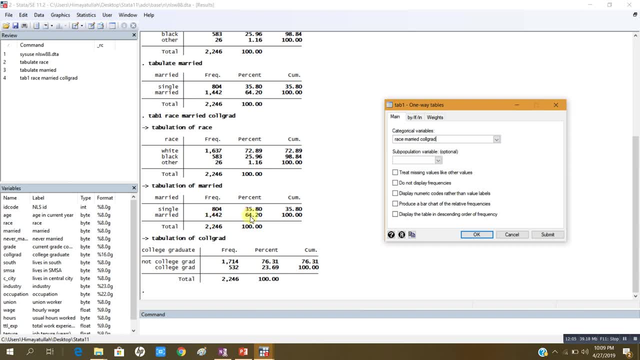 36 percent are single, and this is the one-way classification of college graduates. 1714 are not graduate, not college graduates, 532 are college graduates. so, uh, 76 percent are not college graduate and 40, 24 percent are college graduate. these are their cumulative percentages. now, 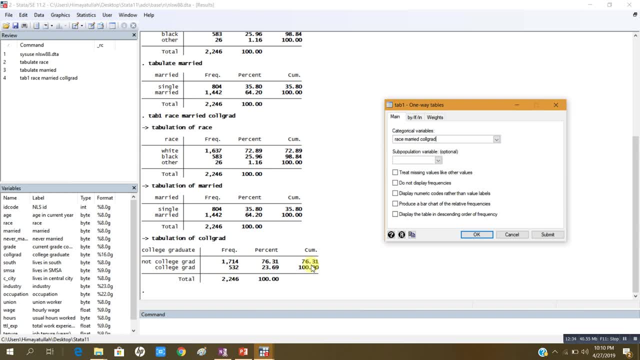 let us suppose now, instead of these three, i want to let me, let me clear all these variables, and i put some more variables in this. let us suppose one is a college graduate and one is south, and let me see if there is any other union. now these are three other. 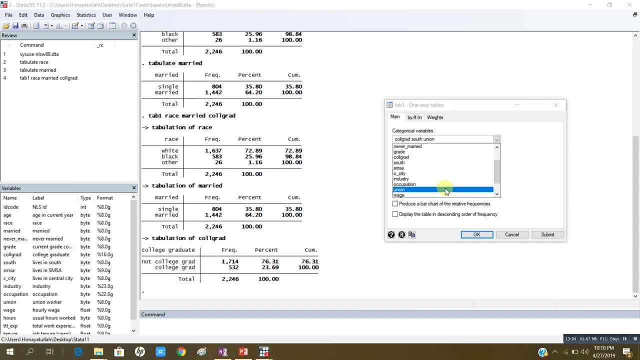 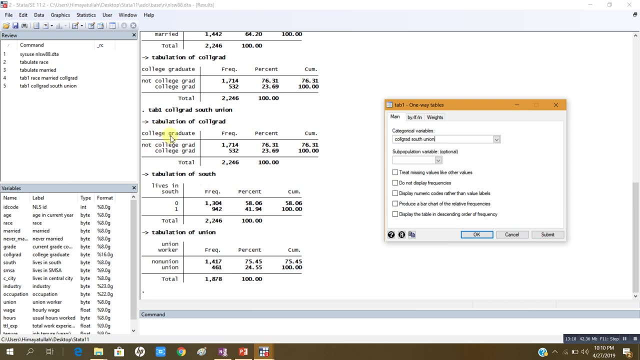 variables and let me submit, submit. let me swallow these variables and let me submit, submit. let me swallow these variables and let me submit, submit. yes, so my first variable was College graduate, and this i already explained: 76 percent are non-colleged graduate and 24 percent are College graduate. 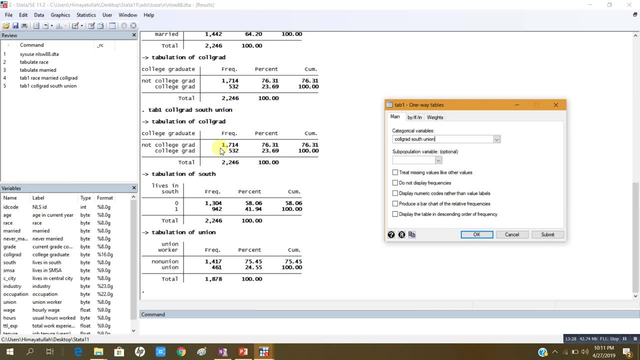 in the second table, 58 percent of the total number of individuals is graduate. 60 Awakening isn't a very difficult. disappeared cleanuum, i expect. okay, let me hurt you that way. sideliness isn't a very difficult yumi, what we will explore till i make due attention to this activity. 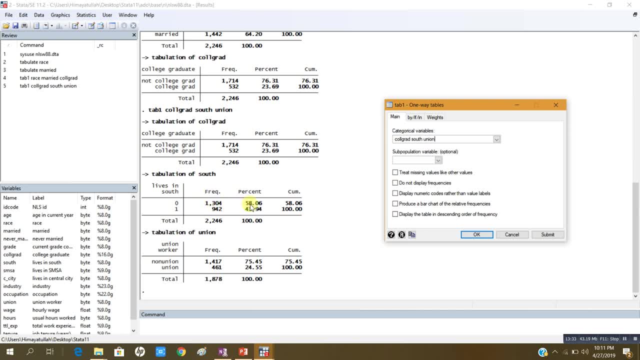 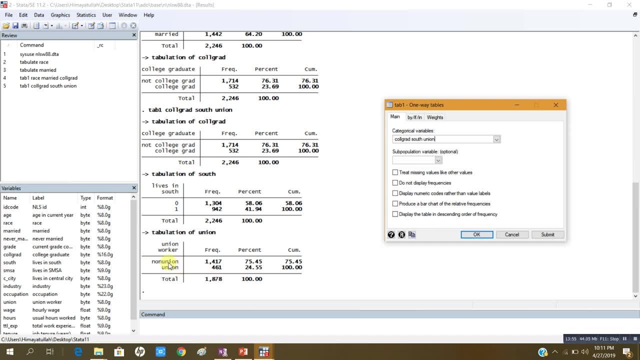 Now, if you look at this table, 75% of them are not member of any union and 25% of them are member of the union. So this is how we classify these variables according to the categorical data, And these are multiple one-way tables. 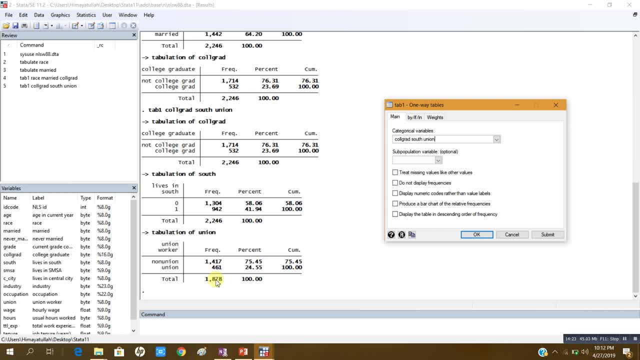 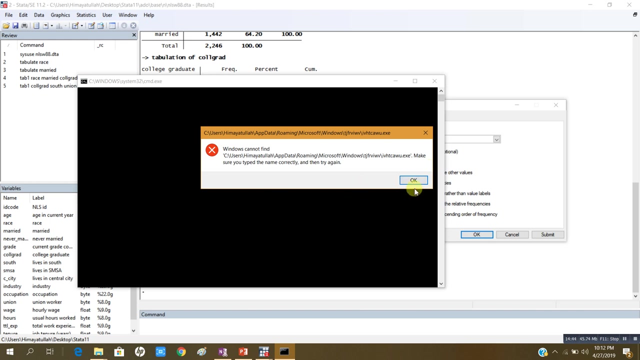 Now I will switch to Another classification, and that should be two-way classification. In these tables you are just having one-way classification of categorical variable. Now I will combine two categorical variables and that analysis will be a little bit different. So let me go to statistics. 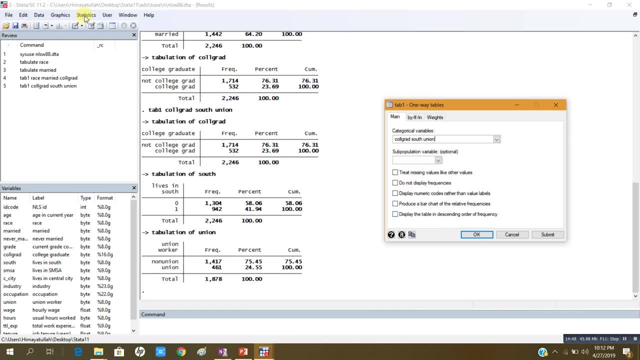 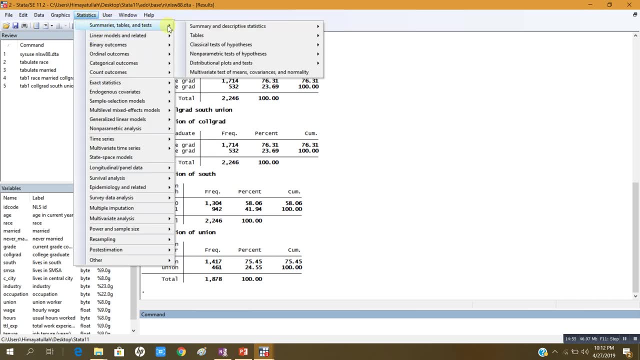 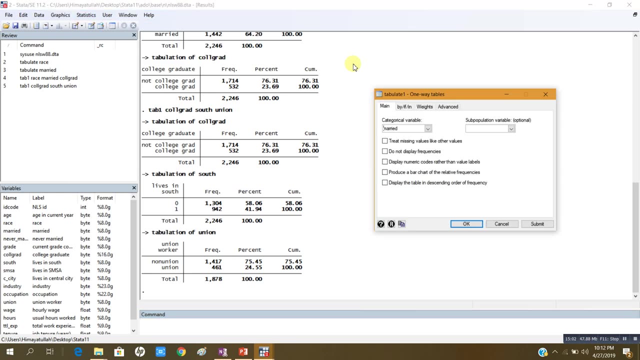 And this time, This time under under table, Under table, Under tables, I will go to two-way tables. Now I'm here And this time it will be: Let me, let me see it again, Sorry. Table Tables, Tables. 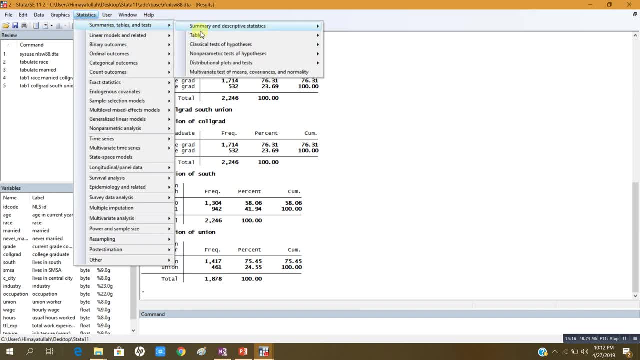 And Two-way tables with measure of two-way And Two-way tables with measure of two-way And Two-way tables with measure of two-way And Table. Table of tables with measure of association. So, So, So. 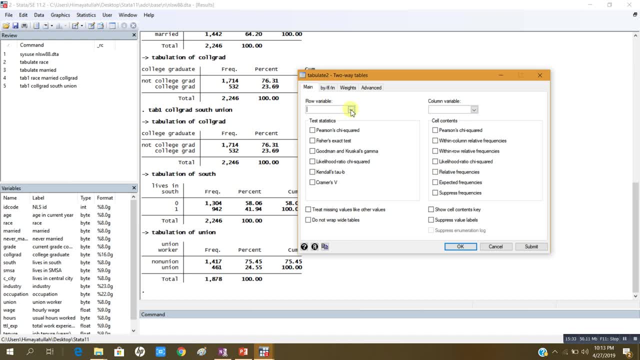 So I want to make a classification Of respondents by And Rates. Rates will be row-wise, row variable and the race will be a column variable. Rates will be a column variable, And let me submit, And let me submit. 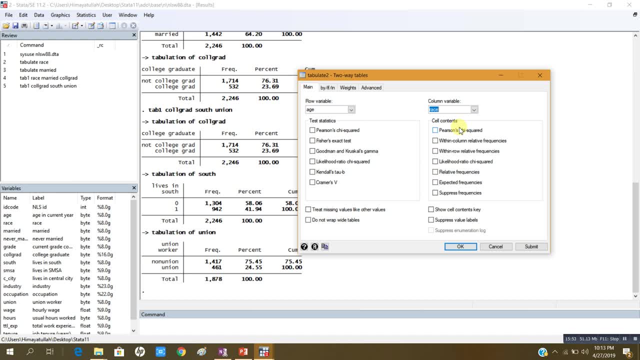 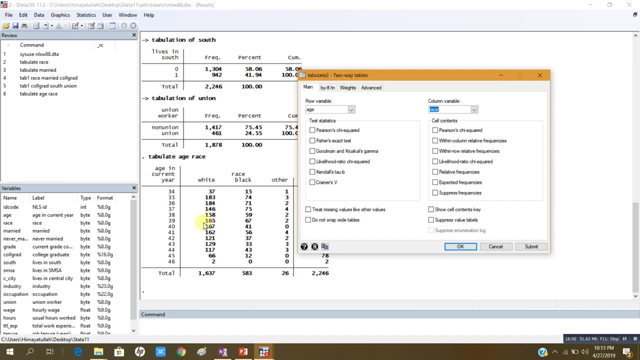 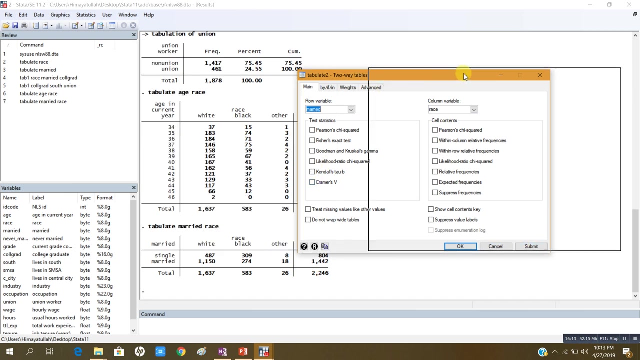 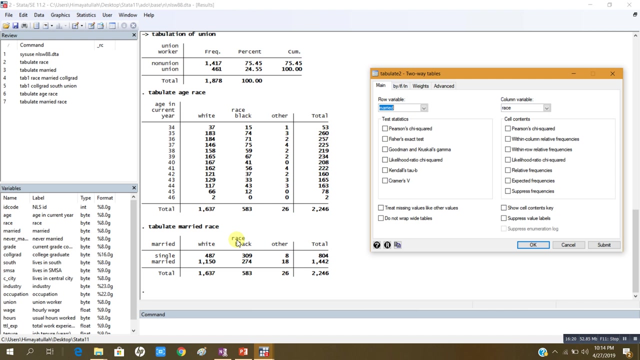 I will press submit. So here is the sorry. sorry, I made a mistake. And instead of age let me put merit here, so that it could be simple. Yes, here it is Merit and race. both are categorical variables. And this is true a classification. You see, row wise, we measure merit, that is, single, or merit, And column wise, we measure the race, that is, white, black and other, And the last column shows total of them. 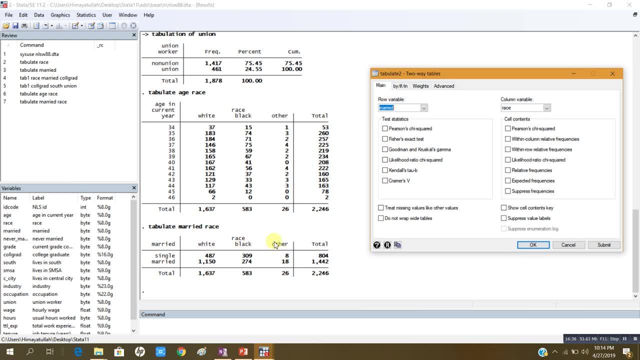 Now, if you look at this, the total number of respondents are 2246.. And out of this total, 1442 are married and 804 are single. Similarly, out of this total, 1637 are white, 583 are black and 26 are otherwise, And this cell that is 487.. This means that these are single white. 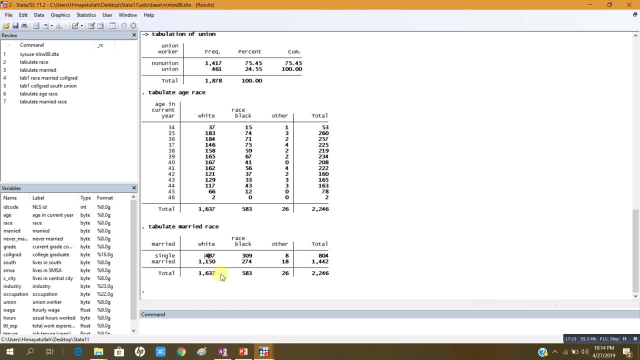 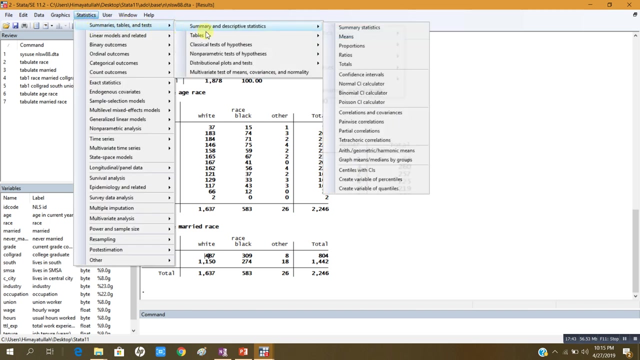 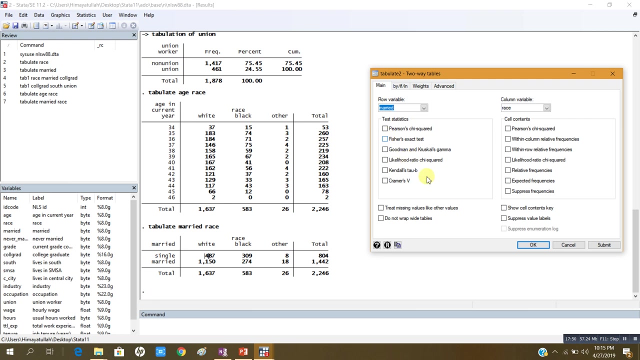 And means white married, 309 are black single and 274 are black married, and 18 means other married which are neither white nor black. now let me check how can I measure association between these two? I was here, let me check person chi-squared, so if I press ok again this, 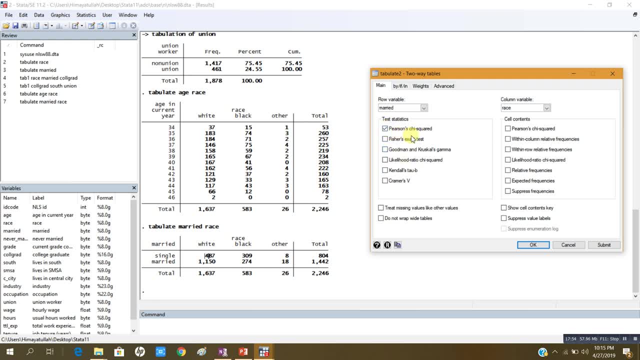 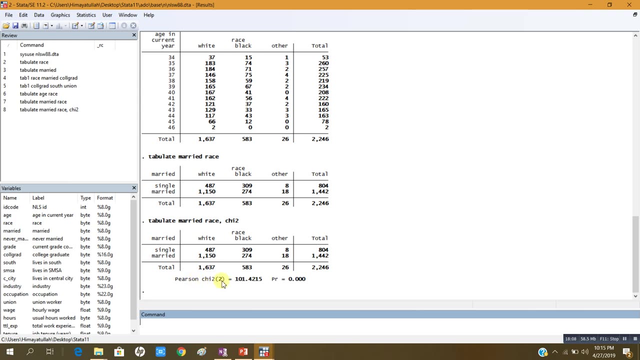 table will appear, but but with the person chi-squared T statistic. so again, table is the same, but this time it has a chi-squared test statistic and issue is 1, 0, 1, point 4, 2 and its p-value is a 0.00. so it means that the null hypothesis of no association between the 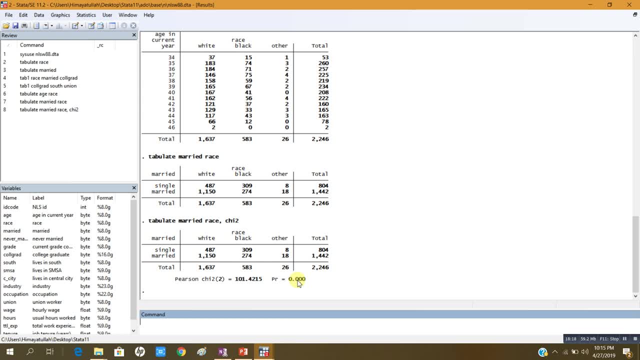 two categorical variable of race and marry is strongly rejected because the p-value is much less than 0.05. so we conclude that there is association between race and marriage. now let me see if I can find the reasons of your interest in our total. that would show you something else. be the. 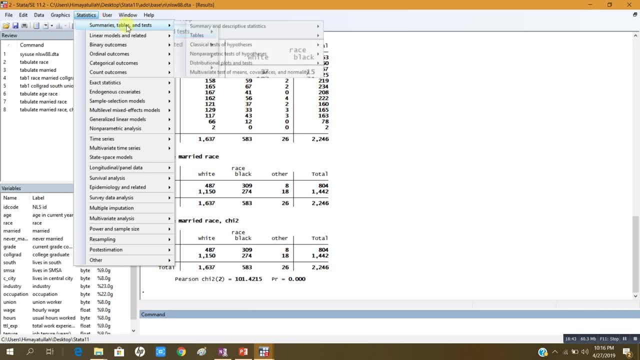 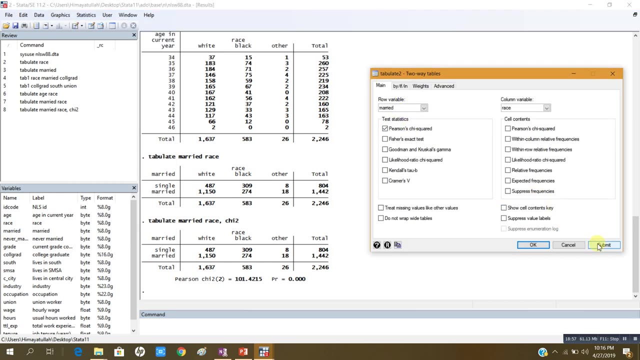 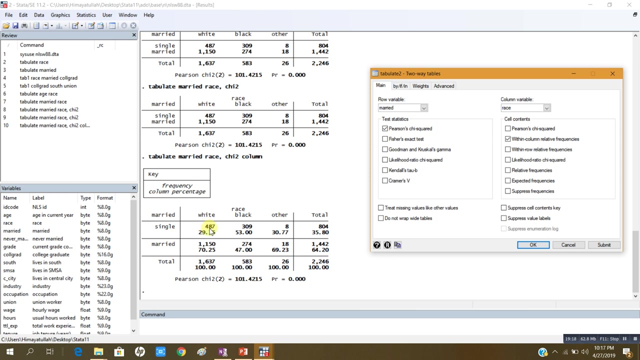 same table. yes, let me submit it first this time and then that in this table i want for transfers, column wise, for I will check this within column relative frequencies and i impress a Submit. So now you see that along with these frequencies, now there are percentages, and these percentages are column wise. Now this is: 29.75 are single white and 70.25 are white merit, and the total is here. 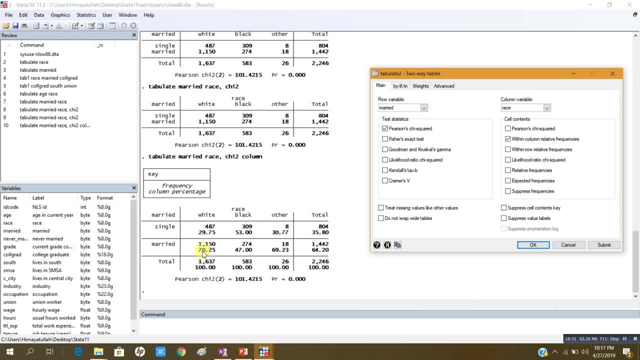 Now there is another column percentage. Here is column percentage and here is column percentage. Now let me make it uncheck this and I will check on within row relative frequencies And if I submit it now, this time the percentages will be row wise. Previously these were column wise, Now these are row wise. 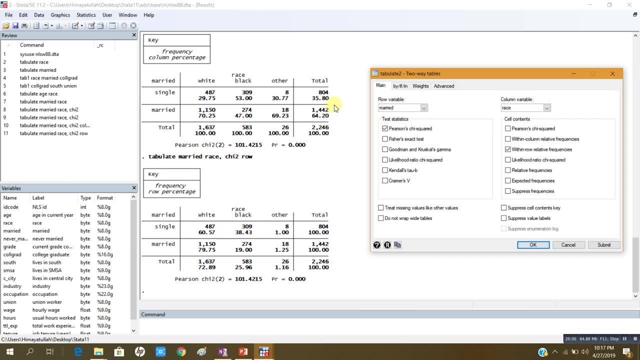 You see, Total is 100 here, and then total is 100 here and total is 100 here. Now I want to see the relative frequency. Now, table will remain the same, but these percentages will change and I will explain what does it mean. Now, this time, these percentages are neither column wise nor row wise, but they are percentage out of this total. 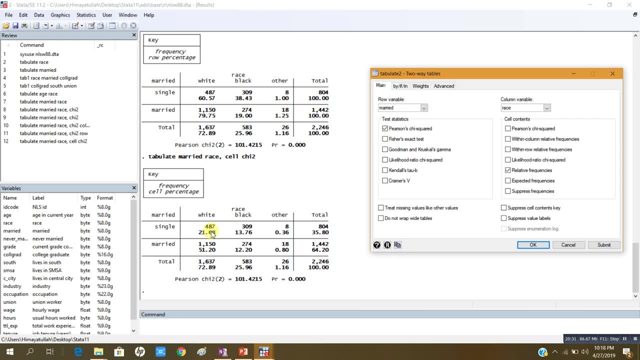 It means that white single are only 21.68% of the total sample of 2246.. Similarly, other single constitute only 0.36% of the total, And here black merit, who are 274 and they are 12.20% of the total. 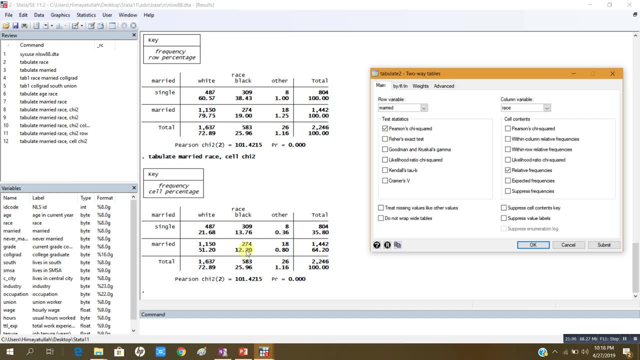 So, ladies and gentlemen, this is how you can make various kind of tables as per your requirement, as per your need, And you can play with this. data is very helpful in this. Now, ladies and gentlemen, let me see how can I compute correlation between two scale variables? So let me go to statistics, and this time, 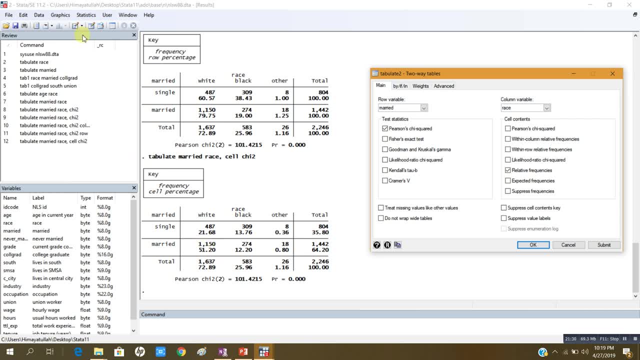 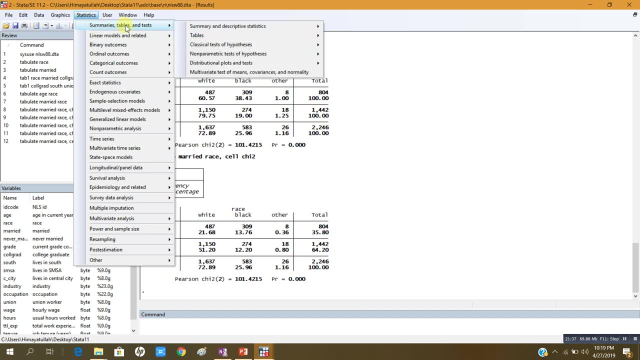 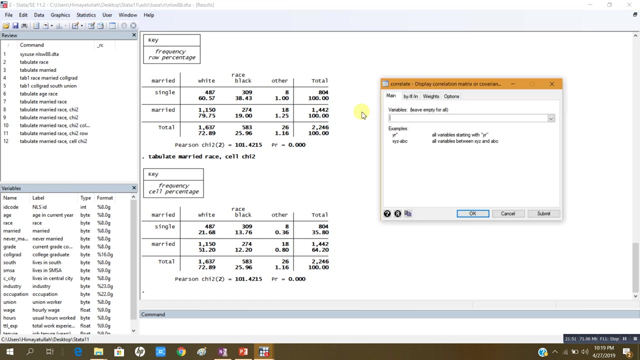 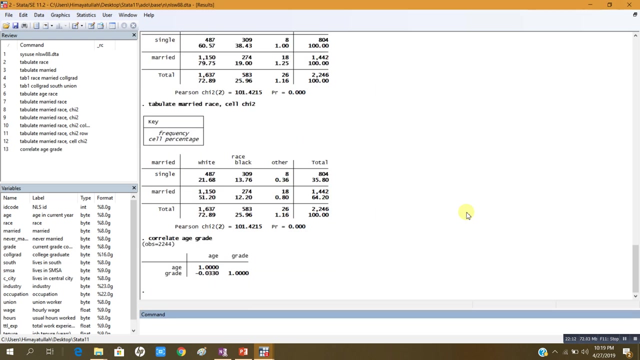 Now, This time I can check for a correlation. Yes, here are the correlations that let me Click on this and I will press an edge. edge is a scale variable and grade is another scale variable. and let me, And now, Let me submit it. and yes, now you see age and grade and there is a correlation coefficient. 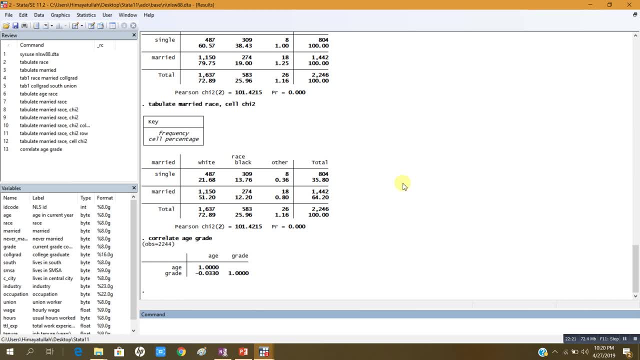 This is the correlation coefficient. This one means that the correlation coefficient of age with age is one. This is positive one, So it means there is perfect positive correlation between age and age. Similarly, this is perfect positive correlation between grade and grade, And this means minus 0.03.. 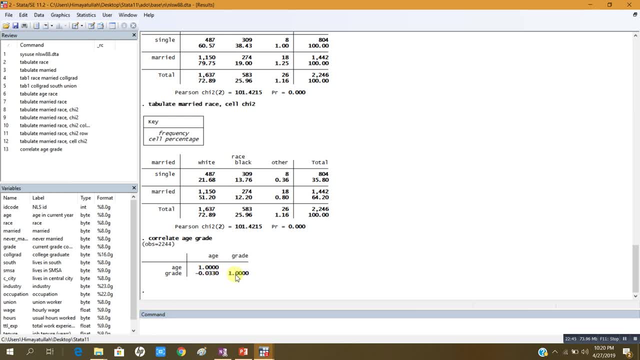 And this is the correlation coefficient between age and grade, And that is negative. It means that age and grade are negatively correlated, Although the correlation coefficient is low, but the sign is negative, So they are inversely related to each other. Now let me see if I can run a linear regression and I will explain it. 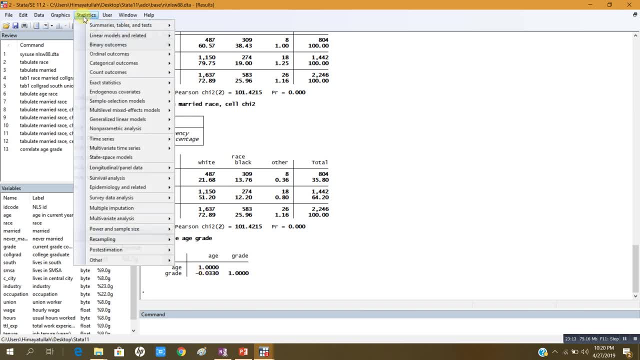 So this time, instead of summary and tables, I will go to linear models and relate it. And here is a linear regression And if I press this I'll get this dialog box. And under this dialog box you see two different things. 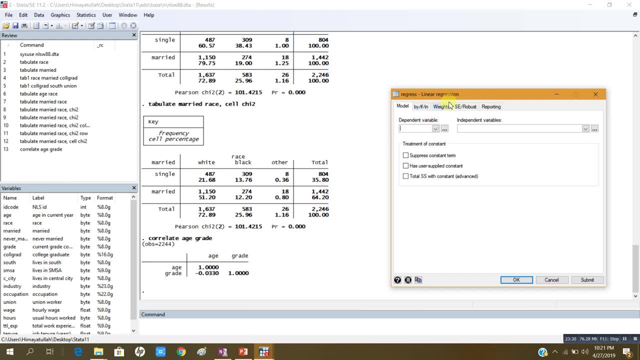 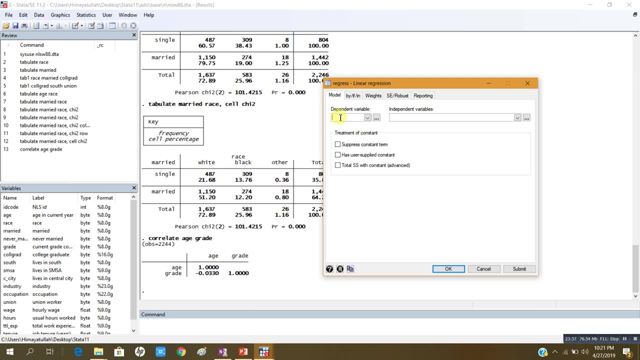 Here is a blank space for dependent variable And here is a blank space for independent variables. Now this space is a little longer because I can include more than one independent variables, But here, independent variable, I will include only one variable. Now let me click on this and there are a number of variables. 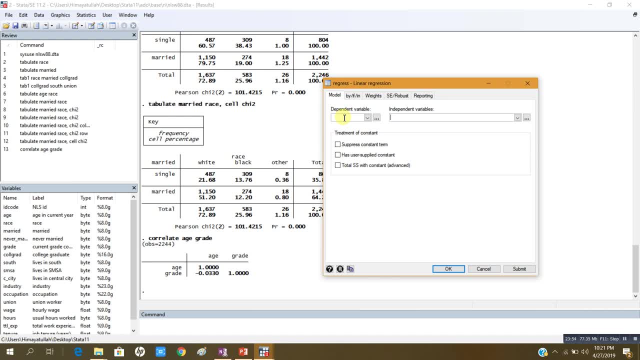 Let me see. Okay, Let me put wage here. Wage is a numerical variable and I want to see what are the independent variables and how the wage depends. So let me click here. Let, First of all, I will include total experience. 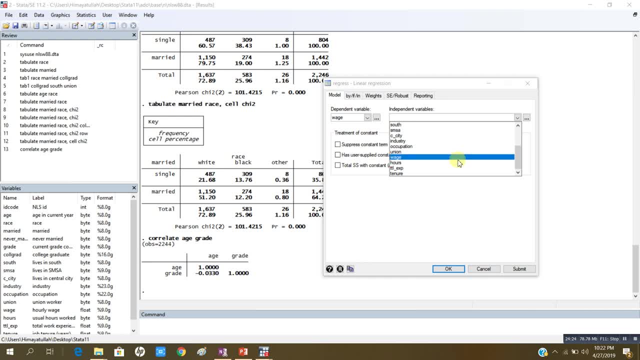 Then 10-hour run job, And then hours worked, And then say union. And let us suppose I also put one more variable name, which is age. So let me submit it, And here are my results. These are my results. And if you look at the command, it says regress. 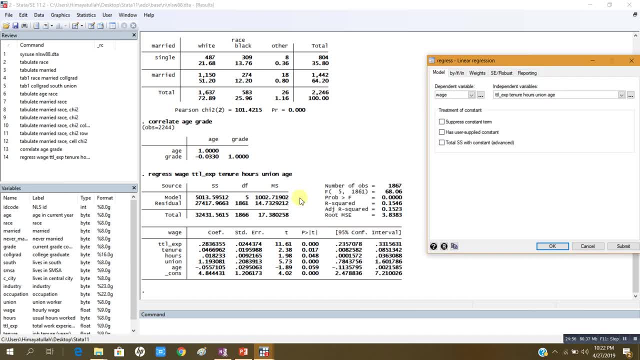 Wage. Wage is my dependent variable And this is total experience. This is work experience on the present job And this is number of hours worked per week And this is membership in the union. that is member or non member, And this is the age. 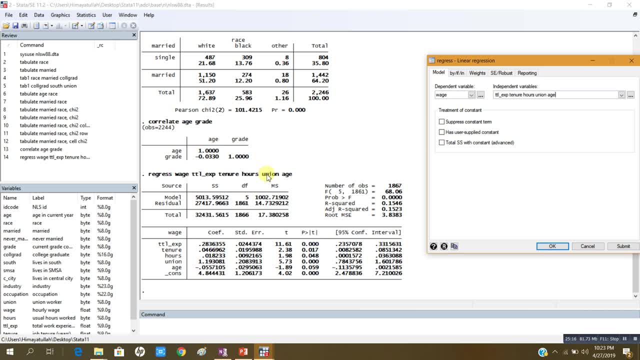 Now this is just like ANOVA And this is a residual. This is regression sum of square. Regression sum of square, or you can say explained sum of square. In front of model and below ss you see 5013.595,. 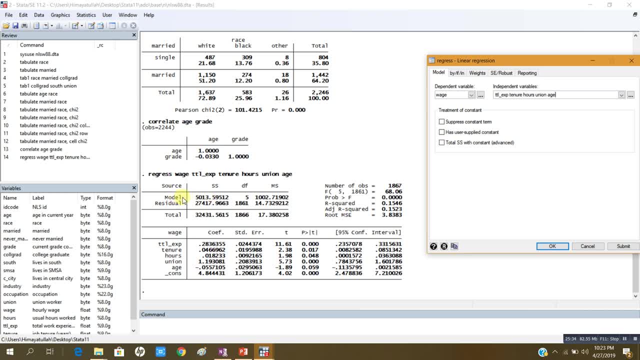 and this is model sum of square or you can say explained sum of square or regression sum of square. Then below this value there is 27,417.97, and that is residual sum of square and this is total sum of square And these are degrees of freedoms and these are mean sum of square and 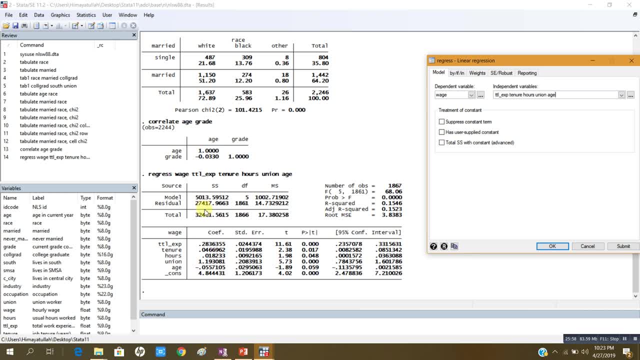 so on, And these are number of observation. total number of observations are 1868.. And this is the f state, which is equal to 68.06.. This is the p value of status f state. this is r squared And this is adjusted r squared And this is rule. this is root mean, sum of mean. 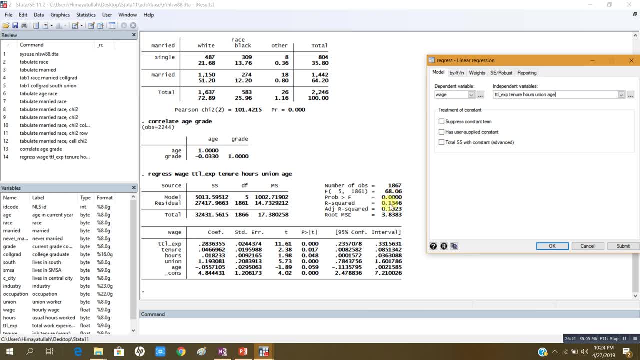 mean square error Here. this table below gives us a number of information. Wage is my dependent variable here, And these are independent variables. Stata by default shows constant at the end of these independent variables. So first variable is total experience, Then there is tenure, then hours worked, then categorical variable for: 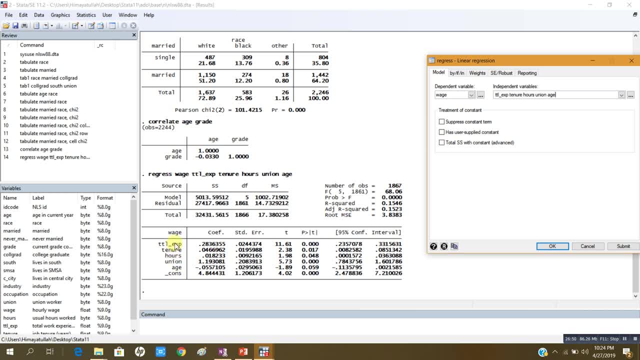 membership of the union, When or otherwise. Age. and these are the numerical coefficients of these independent variables. These are the standard errors of these coefficients. These are the t values And these are the p values And if you look at this table, by coincidence, all included variable in this model are significant. None of none of them is a. 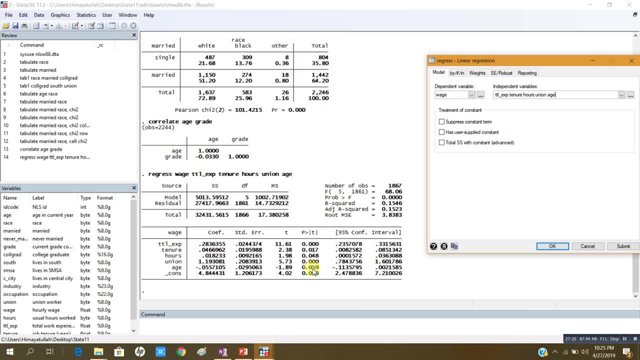 significant except a age. but if we, if we assume that the alpha is equal to 0.10, then this is also significant. otherwise, at 5 percent level, except age, all other variables are significant. and here is the, here is the 95 percent confidence interval. now, this means that if total experience increases by one year, 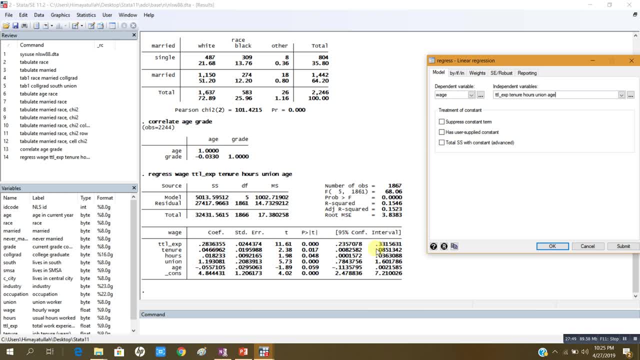 then the wage increases by, say, 28 cent per hour and similarly, this is the coefficient after never. if on the present job the experience increases by one year, then the wage increases by 4 cents per hour. and these are our work. these are also positively rated and this means that if a person 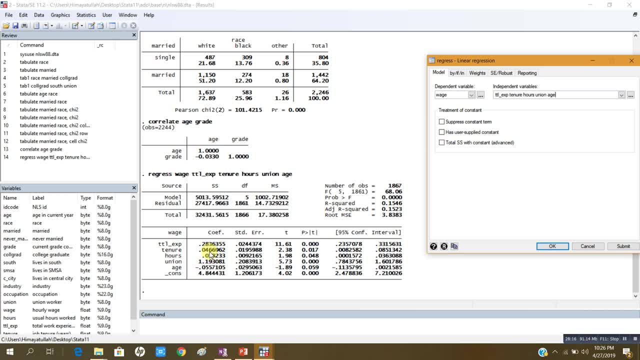 is a member of the Union, so he's a is hourly wage is higher by one point one, nine dollars, as compared to a non-member, and it has a negative relationship with age, that is, with every year of age the wage per hour wage increases by 0.05 cents. and this is the intercept. ladies and gentlemen, this is sufficient for today. this. 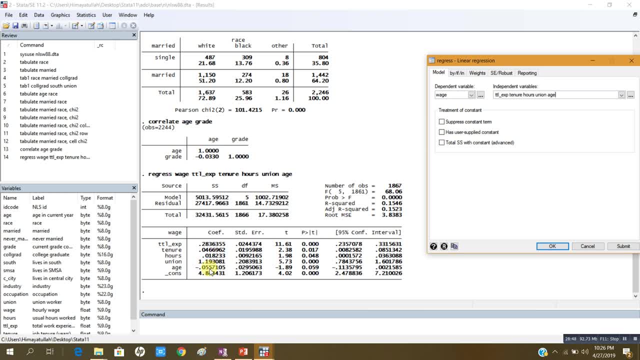 is the very basic video on Stata. I just started data analysis with the Stata from tonight and I'll continue it slowly in grind, Gradually. I will use elementary and then intermediate and then advanced level a data analysis with Stata. I hope you will learn with me and you can share. 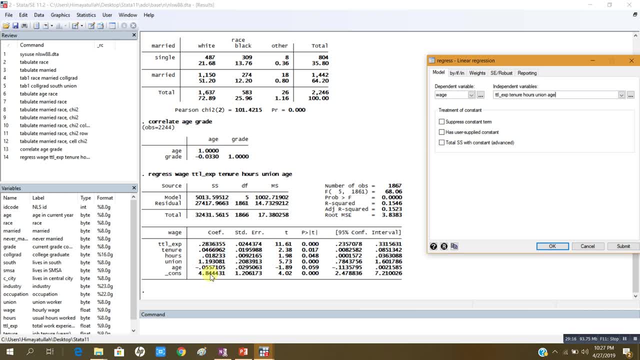 you this video with your friends, with your colleagues. here is your Google Mageos tutorial and you'll also get. and, gentlemen, if you haven't yet subscribed to the channel, kindly do so and don't forget to click on bell icon so that you can get notification about my other videos. thank you very much and have a. very good night. 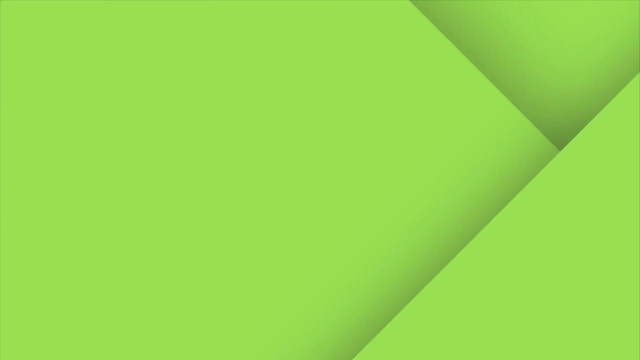 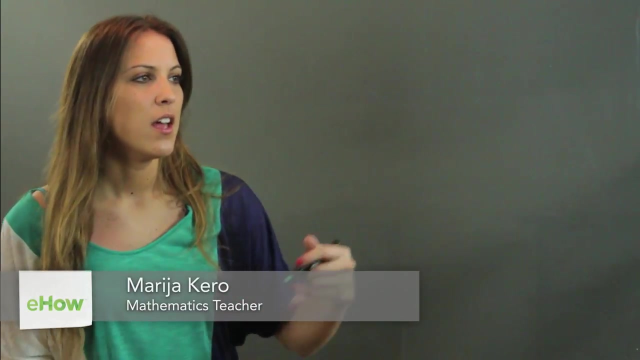 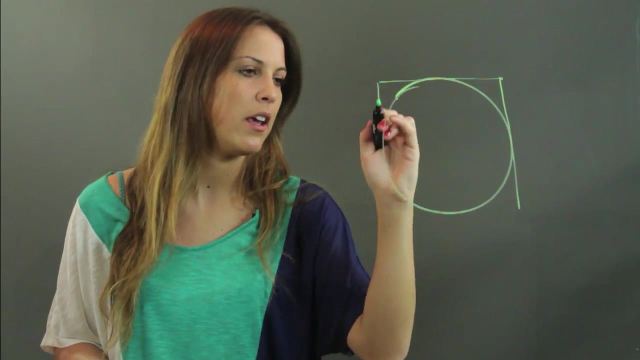 Hi, my name is Maria, I'm a mathematician and today I'm going to show you how to determine the length of a square by using the diameter. So if we have a circle that is inscribed in a square- and you're going to have to kind of pardon my drawing- and we know the length, 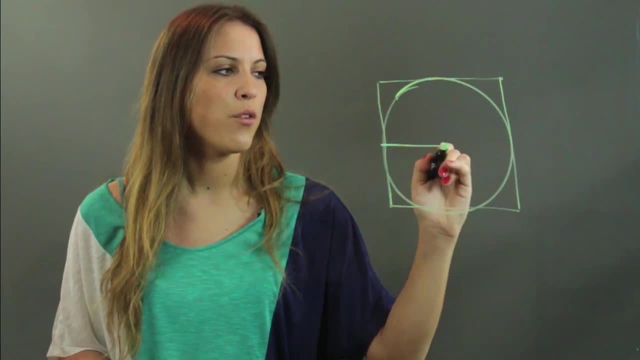 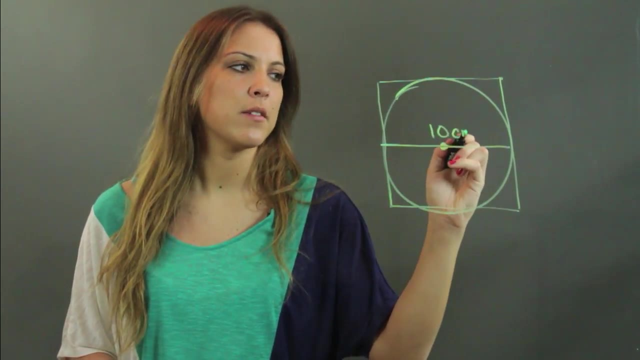 of the diameter. So the diameter is a line that goes from one end of the circle to the other, going through the center. So let's say the length of that diameter is given to us and it is 10 centimeters. Well, the length of the diameter is going to actually just 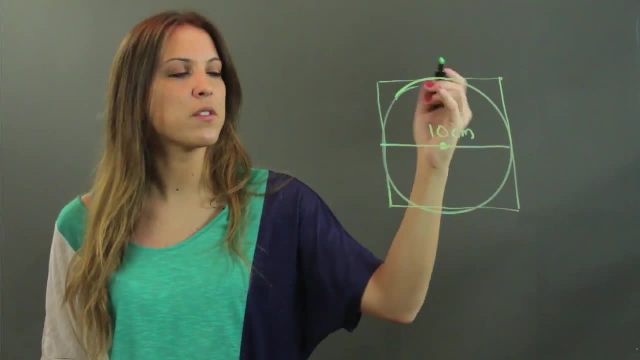 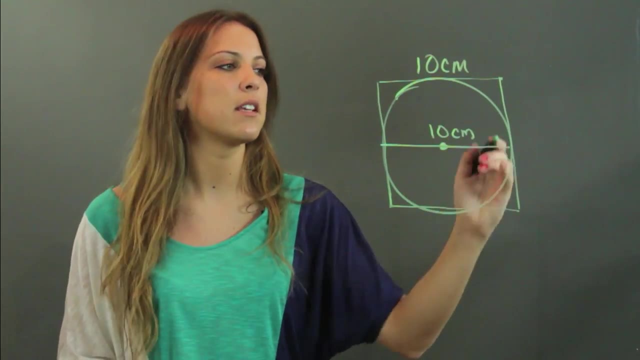 be equal to one side of the square. So if the length of the diameter through the circle is 10 centimeters, then the length of the top of the square has to be 10 centimeters. But then I know that a square has all equal sides. so if that's 10 centimeters, then this: 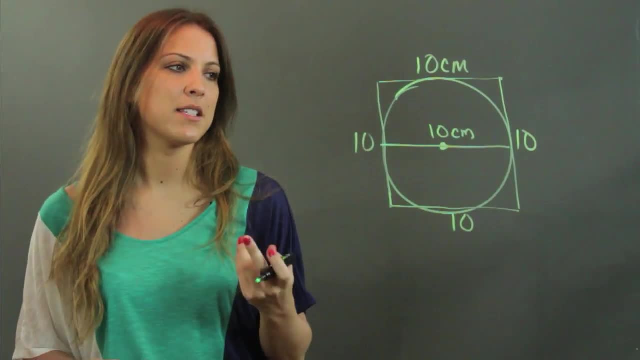 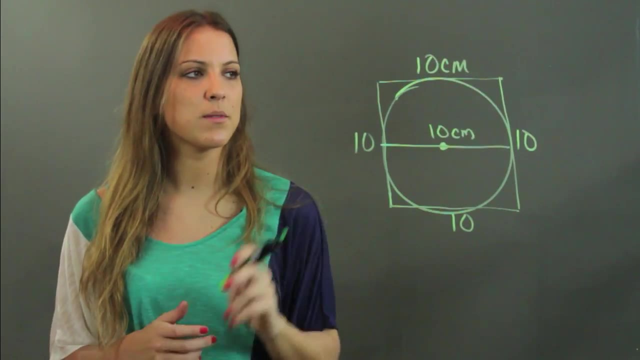 also has to be 10, and so does this and so does this. So now what happens is, if I want to find my perimeter, I just add all the sides up, and I know that my perimeter is 40, or I can just multiply this by four sides. So 10 centimeters times four is 40 centimeters.